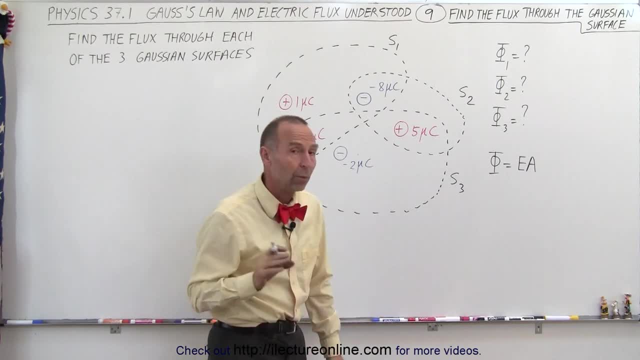 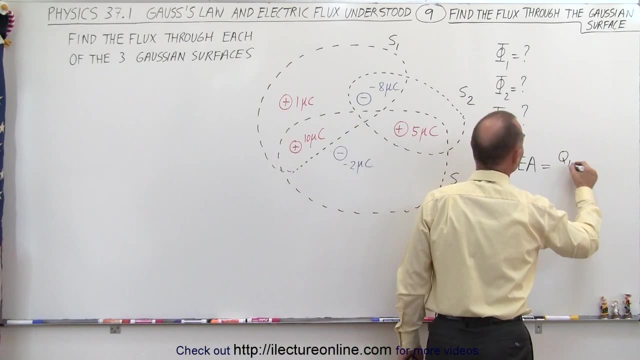 There's no symmetry there. There's no way we can figure this out. However, we also know that, using Gauss's law, this must be equal to Q inside divided by epsilon sub naught, In other words, the flux to any of the surfaces. 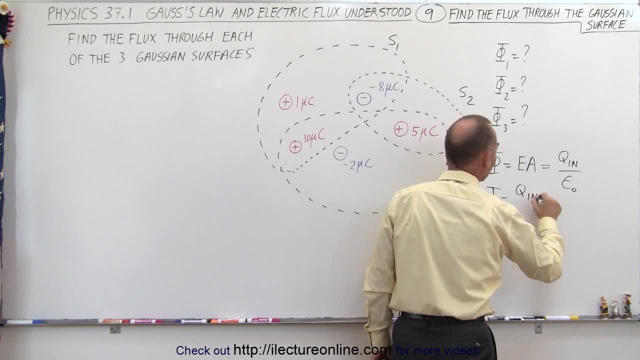 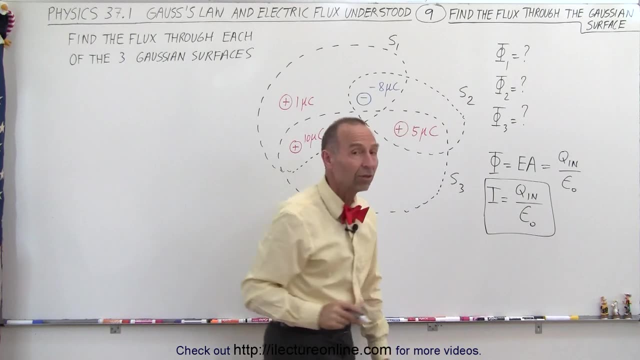 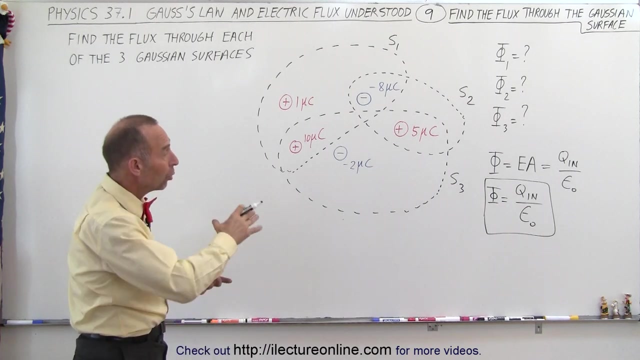 Only depends upon the charge enclosed by the flux, by the, by the Gaussian surface and divide by epsilon sub naught, which is a constant. So all we need to do- and of course any little circle there, there's phi. So all we need to do is simply sum up all the charges inside each surface divided by epsilon sub naught and we have the flux to each of the three surfaces. 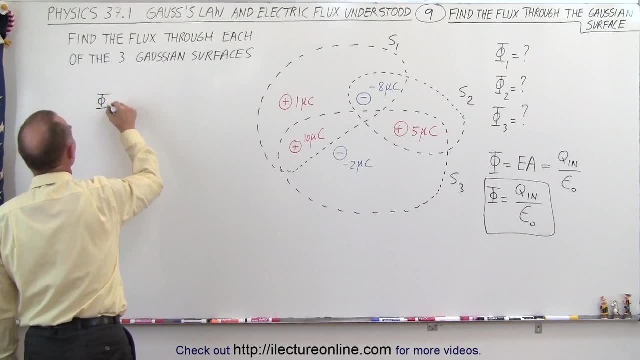 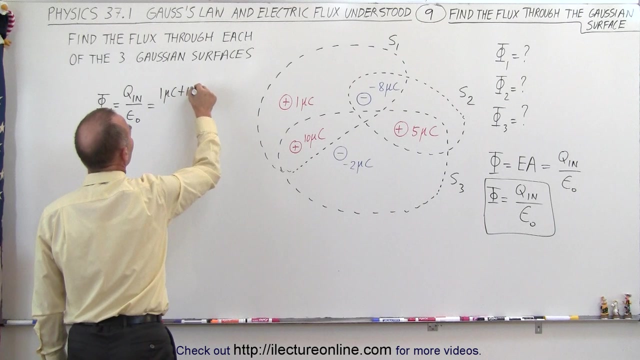 So let's start with surface one. So flux one is equal to The sum of all the charges inside divided by epsilon sub naught. So in this case, for surface one, we're going to add these three together, So that would be one microcoulomb plus 10 microcoulombs minus eight microcoulombs, all divided by epsilon sub naught. 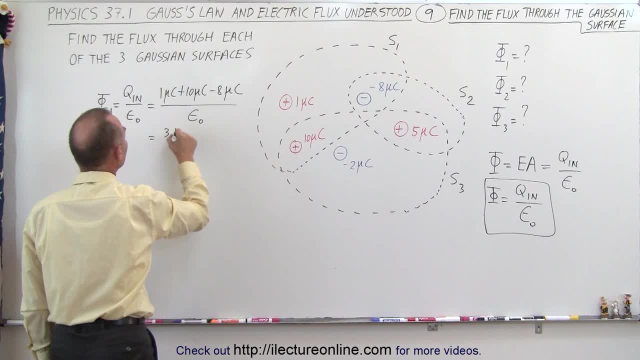 And so this is equal to 11 minus eight, which is three. microcoulombs divided by epsilon sub naught would be 8.85 times 10.5.. To the minus 12, that would be coulombs squared divided by Newton meters squared. 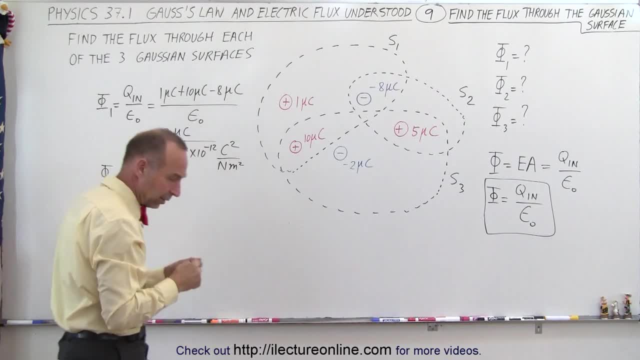 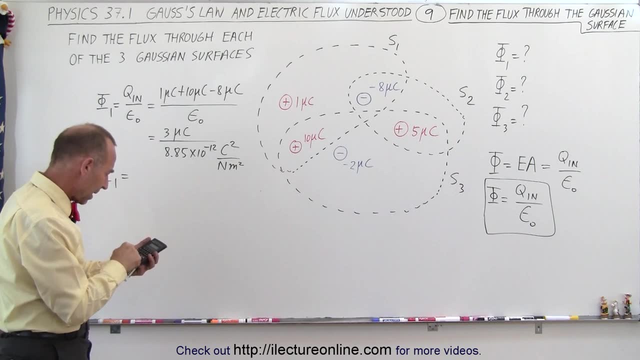 So for the first one, what do we get? So we have three microcoulombs, which is three e to the six minus divided by 8.85 e to the 12 minus equals, And let's see here That's 339,000.. 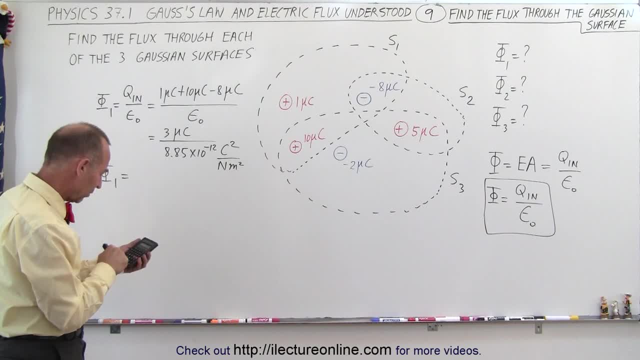 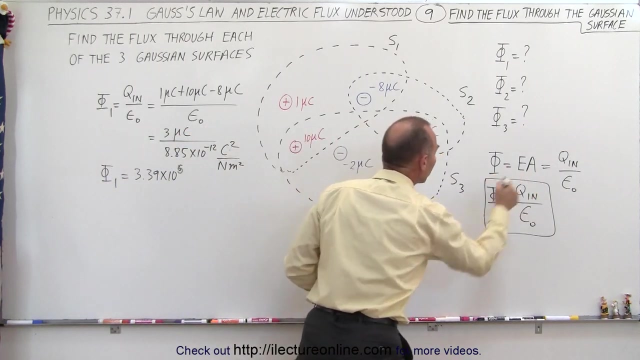 Let me try this one more time. Just make sure: three e to the Yes, indeed 3.39 times 10 to the sixth. So that would be equal to 3.39 times 10 to the sixth, And of course the units would be newtons per coulomb, times meters squared. 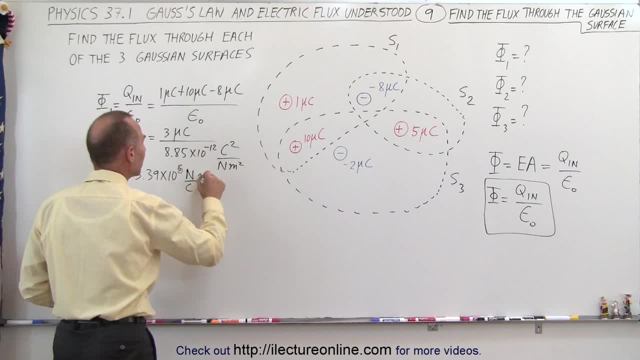 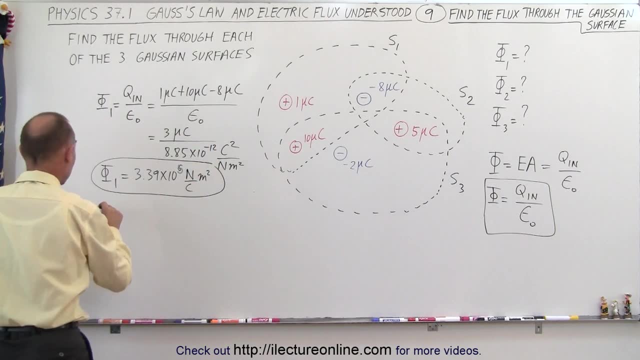 So that's newtons per coulomb times, meters squared, And that would be the flux to the first surface. Now let's do this again for the second surface and see what we get. So flux to the second surface. So flux to the second surface is equal to Q inside of epsilon sub-naught. 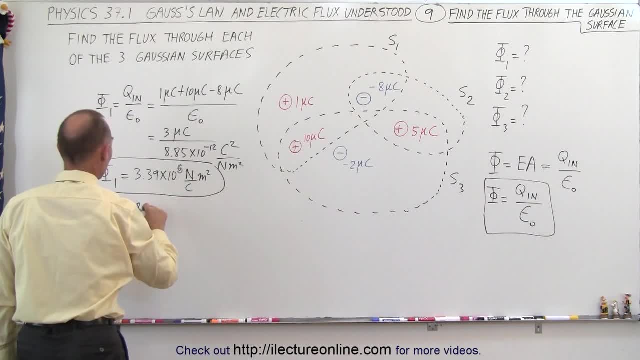 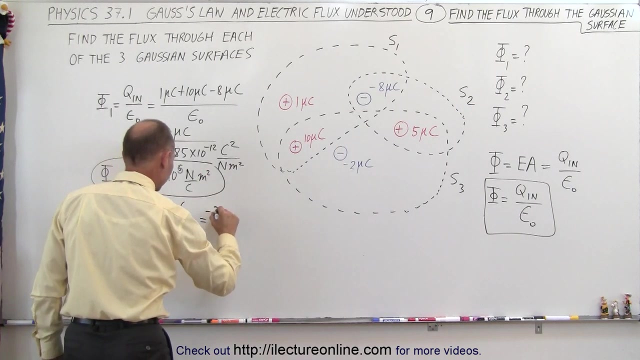 So that would be the sum of those two. So minus eight microcoulombs plus five microcoulombs, divided by that would be epsilon sub-naught, And so this is equal to- and let's just combine the two, That would be minus three microcoulombs divided by 8.85 times 10 to the minus 12.. 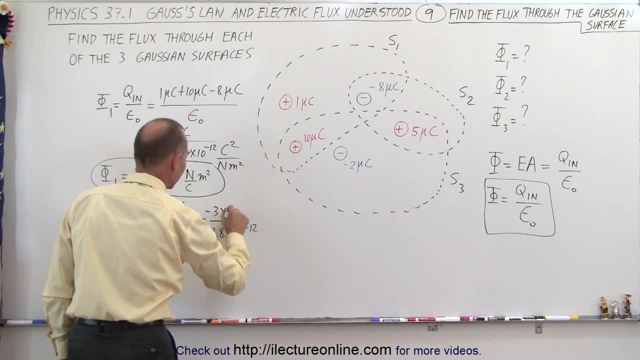 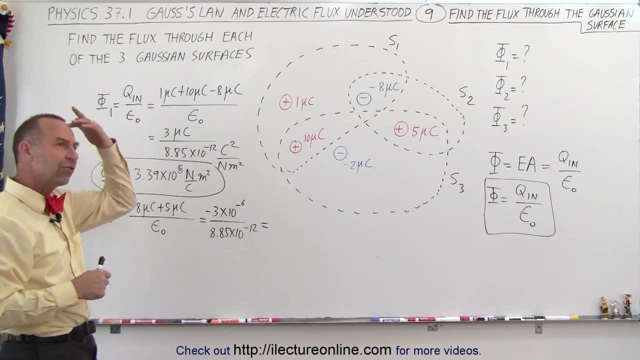 And what I'm going to do here is simply write: That is, S3 times 10 to the minus six. Now you say: well, wait a minute, You have a negative there, negative charge. Can you have negative flux? Well, it turns out, no, there's no such thing as negative flux. 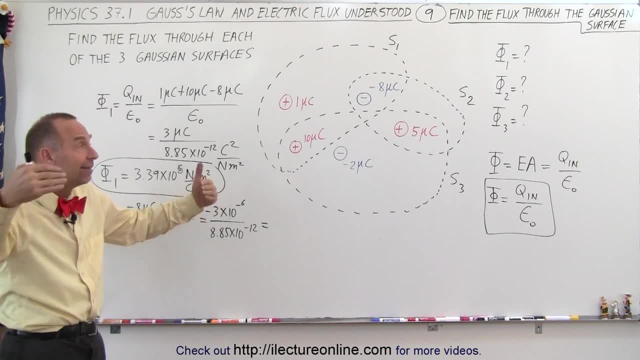 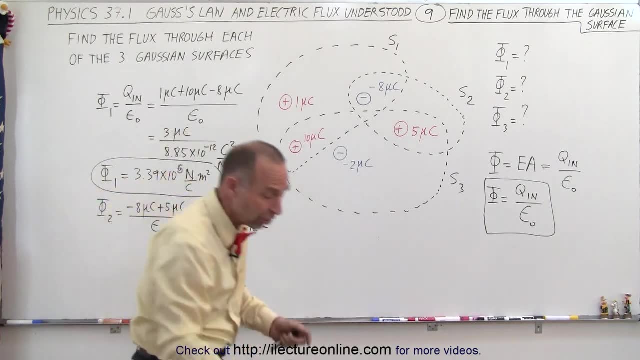 What it does indicate, though, is that the electric field is, in general is, into the surface rather than out of the surface, So that's what the negative means, But, in essence, there's no such thing really as the negative flux. 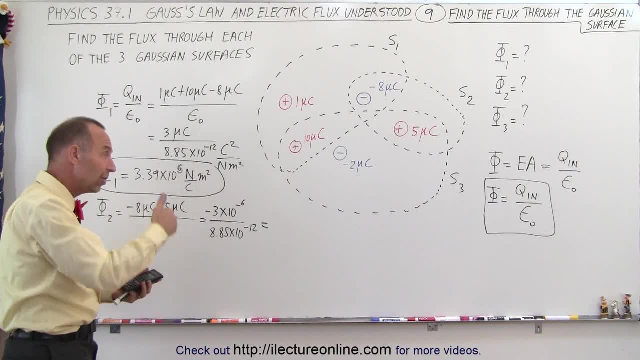 Just the indication. The negative just indicates. The negative just indicates that the flux is in an inward direction. So let's do this one. So it's three: e to the six minus divided by 8.85. e to the 12th minus, which is equal to wow, exactly the same. 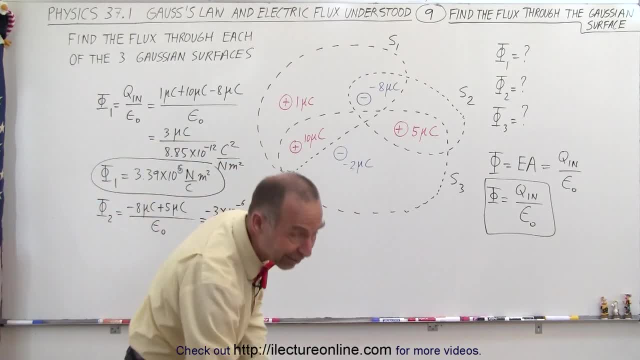 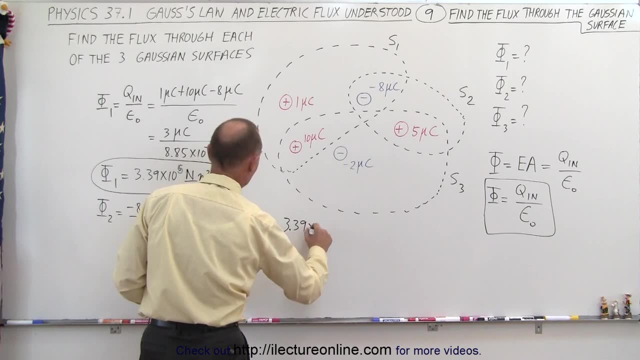 Well, it has to be the same because the magnitude is the same. I didn't even realize that. So we end up with a negative 3.39 times 10 to the sixth. That would be newton per coulomb times meter squared. 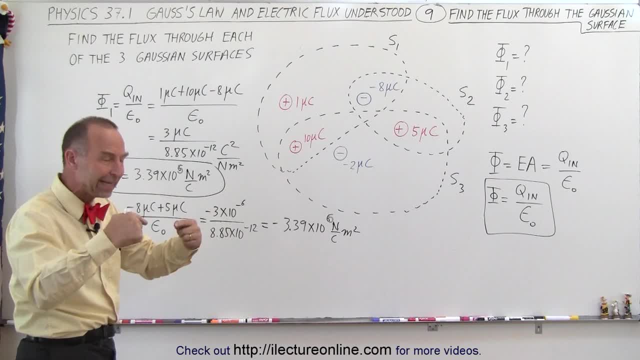 And of course the negative simply indicates that the flux is in instead of out the surface. And then for flux 3, that is equal to: we add all the fluxes together, all the charges together, so it's 10 microcoulombs. 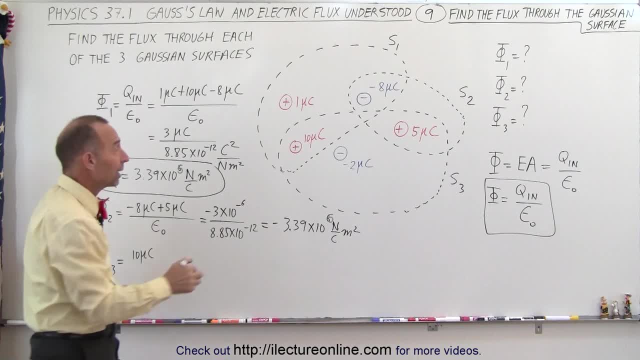 In essence, adding all the flux together would be okay, correct, because we could do it separately. We can calculate the flux for each of the three charges and simply add the flux together. We could have done that as well. So we have 10 microcoulombs plus 5 microcoulombs. 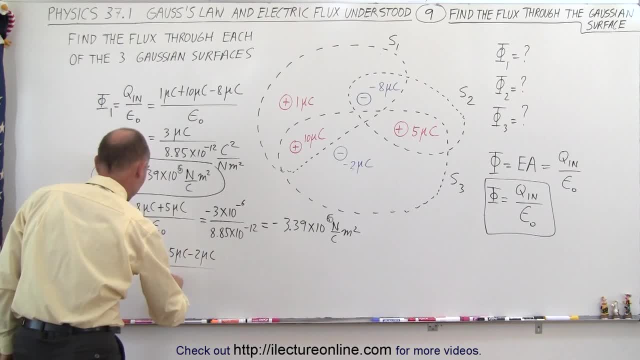 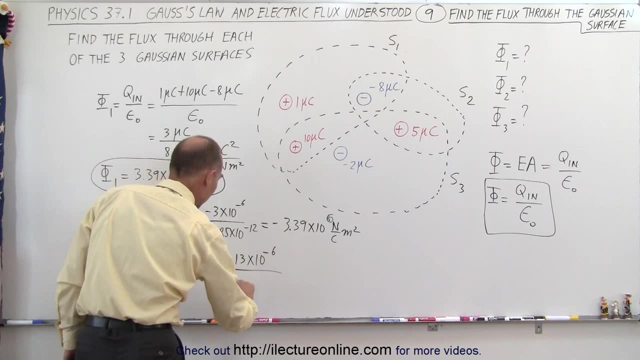 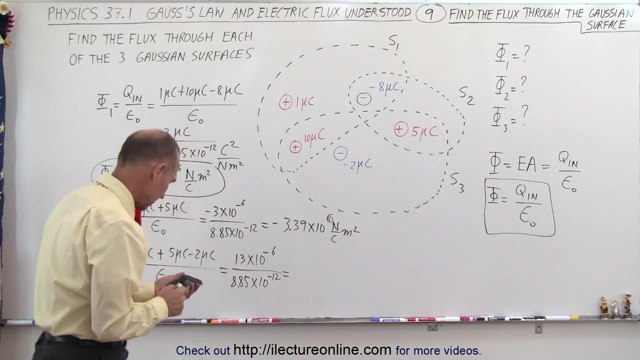 Minus 2 microcoulombs divided by epsilon sub naught. So this is equal to 13 times 10 to the minus 6, divided by 8.85 times 10 to the minus 12.. And let's see what we get here. 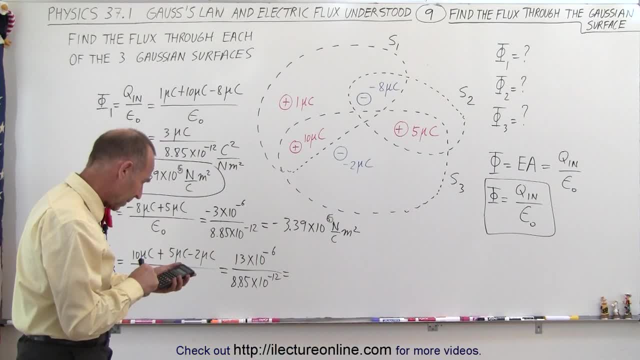 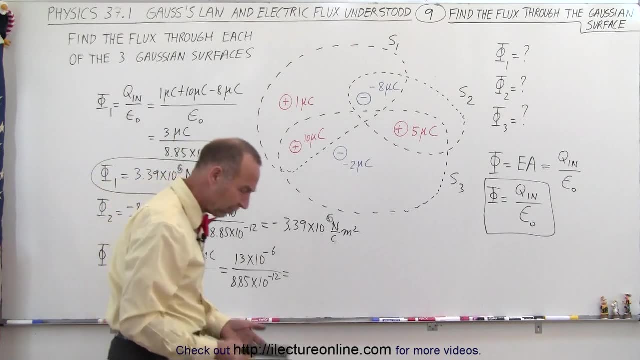 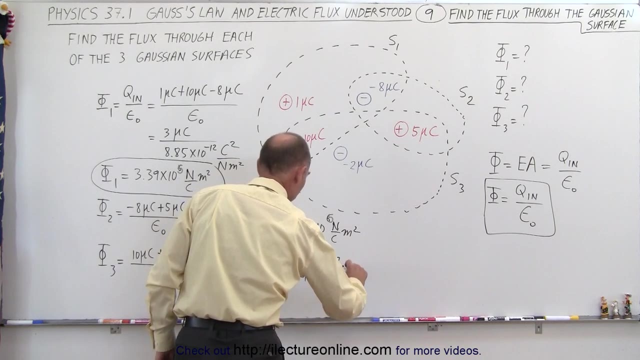 So 13 e to the sixth minus divided by 8.85 e to the 12th minus is: And that would be 1.47.. So 1.47 times 10 to the 7th newtons per coulomb. 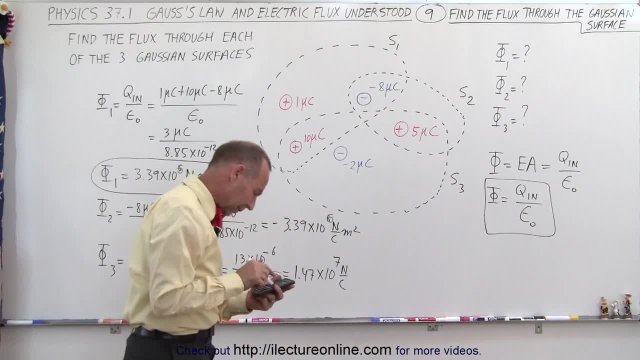 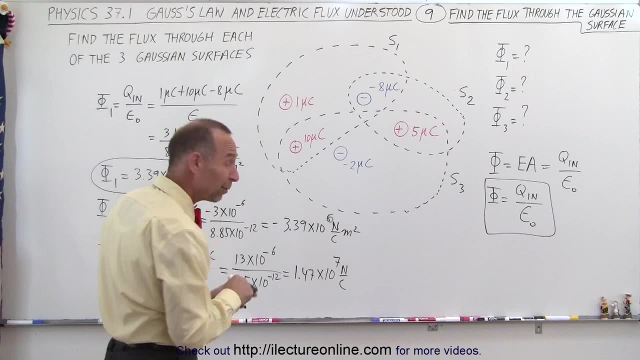 Am I doing that right? Times 10 to the sixth. Let me take a quick look here. Let's see There we go: 1.46.. I think I was off by a factor of 10.. I think these are to the fifth power, not to the sixth power. 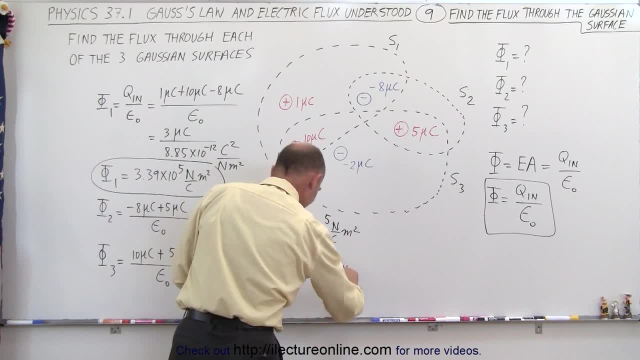 So let me check that in just a moment Again. my eyesight is not as good as it used to be And I don't always see. I see the decimal point, but that's 1.47 times 10 to the 6th newtons per coulomb times meters squared. 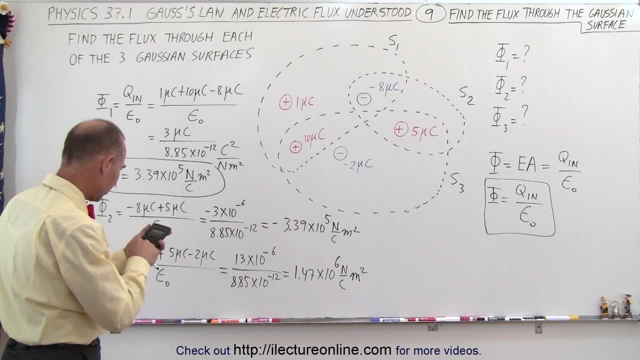 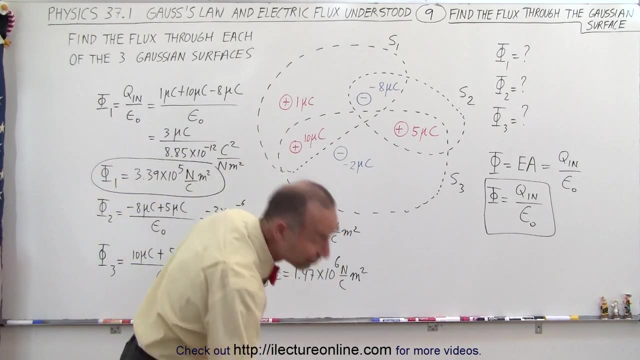 Let me quickly do the other calculation again to see what I got here. So 3 e to the sixth minus divided by 8.85 e to the 12th minus equals. And yes, indeed, that would be 3.39 times 10 to the fifth, not times 10 to the sixth. 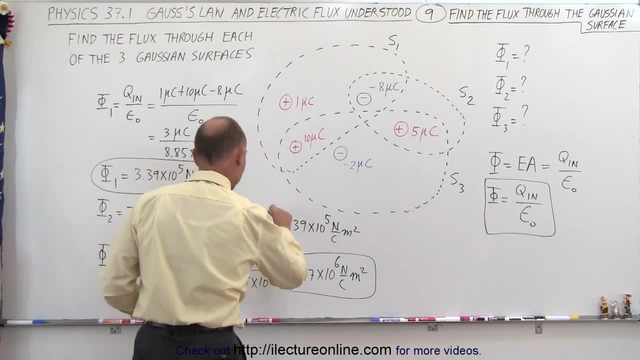 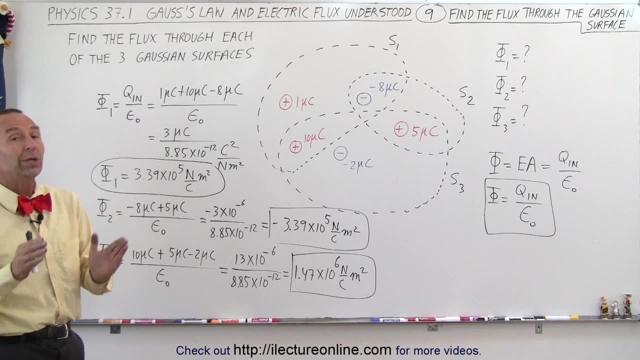 So good thing that I caught my mistakes, Mistakes. So here are the results of the three calculations to find the flux to the surface. So all we need to know is simply what the charge is inside the Gaussian surface to figure out the total flux. 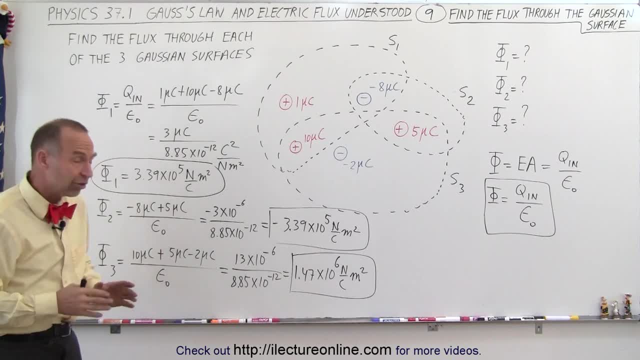 And it doesn't matter the shape or where the charge is, or how close or far away the charge is from the surface. None of that matters. Just the total amount of charge inside the surface is what matters to find the flux to the surface And that's it.